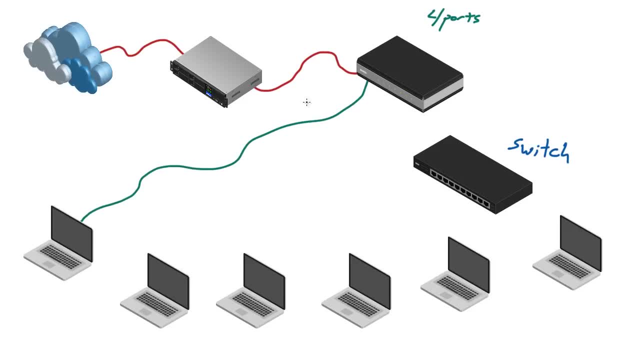 So, for the first three, what we're going to do is we're just going to hook these up directly to the laptops. One, two, three- these bad boys are online Now that fourth port- instead of taking it and hooking it up to another device. what we're going to do is we're going to take this. 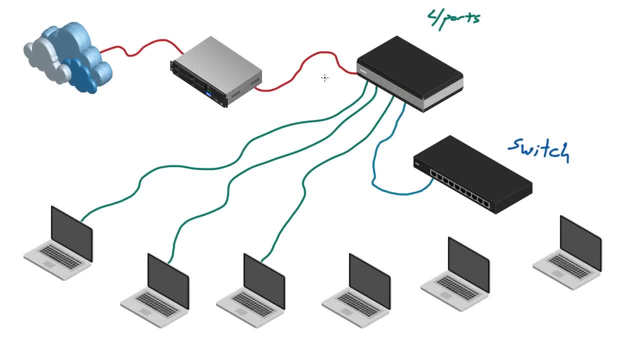 and hook up the Ethernet cable to the first port in the switch, And then what we're going to do is we have all of these extra ports that can now be used for additional devices, So we can take another Ethernet cable, boom, boom. 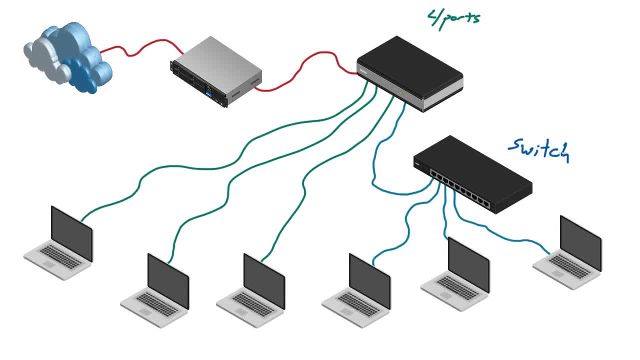 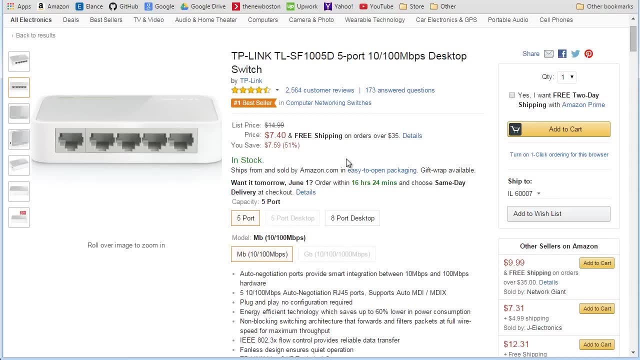 and boom. so check it out. So again, that is what a switch is, And let me pull up a switch and show you guys what it looks like in real life. All right, so this is just the first one. I found It's the number one best seller, the most popular one on Amazon. 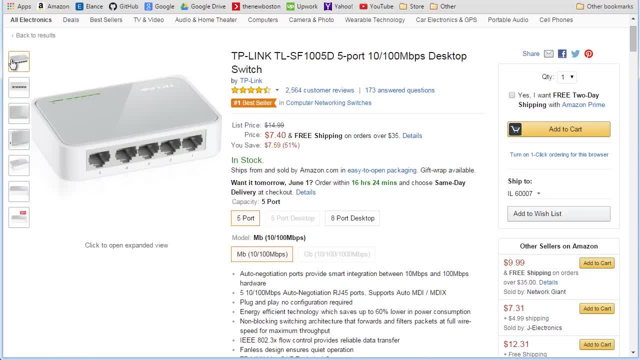 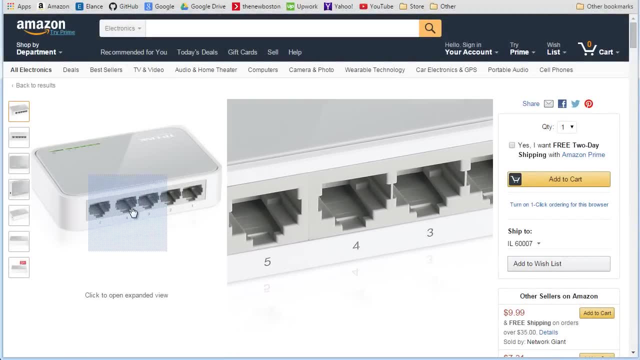 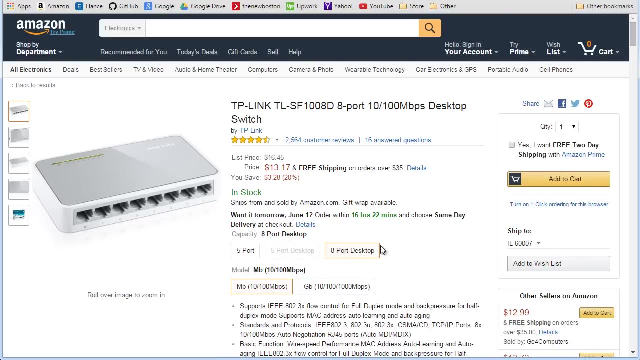 And again, this is what it looks like in real life. And, of course, this right here is a five port switch. One of these has to be devoted to the router. The other four can be used to hook up additional devices. You can also choose to get a switch with more ports, but those are more expensive. 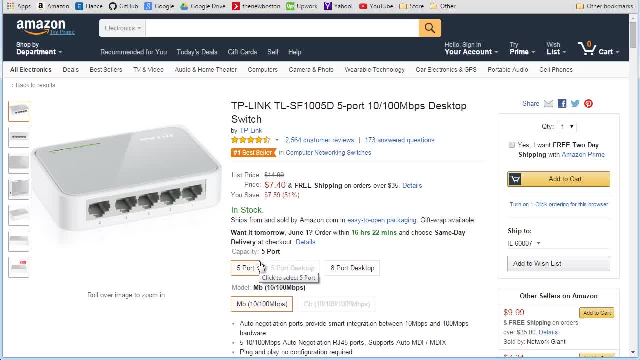 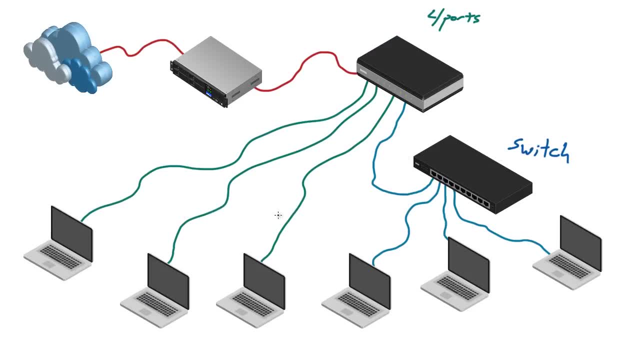 Depending on your need. choose however many ports you want. And also, you're probably going to see the words unmanaged and managed as well whenever you're looking at switches. Whenever you see the word unmanaged, this means that you can pretty much just take it right out of the box, plug it in and it's going to work. 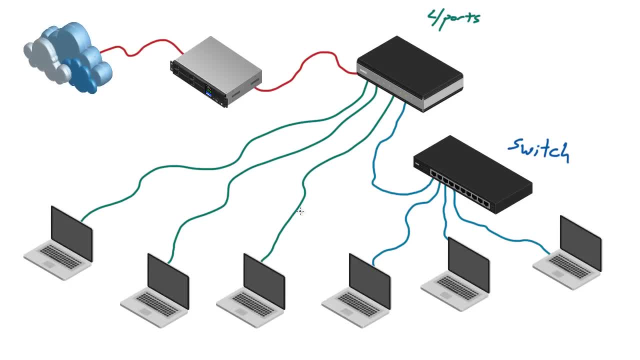 Whenever you buy a managed switch, this just gives you some more settings. It allows you to monitor the network, Maybe alert you when something goes wrong. It can tell you which parts of the network are used more than others. So if you just need something really simple to connect more devices, then just buy an unmanaged switch. 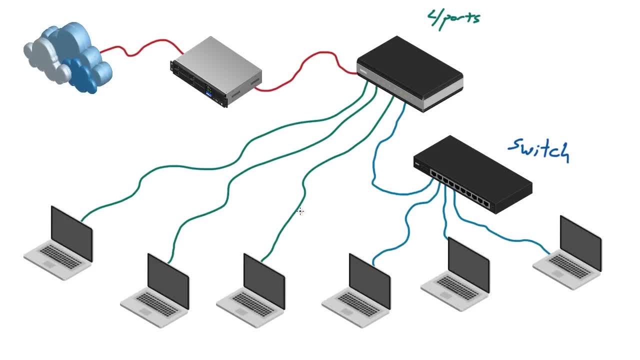 But if you want a little bit more control over your device, then buy a managed switch. And yeah, there you go. That's the basics of what a switch is. I'll see you next video.